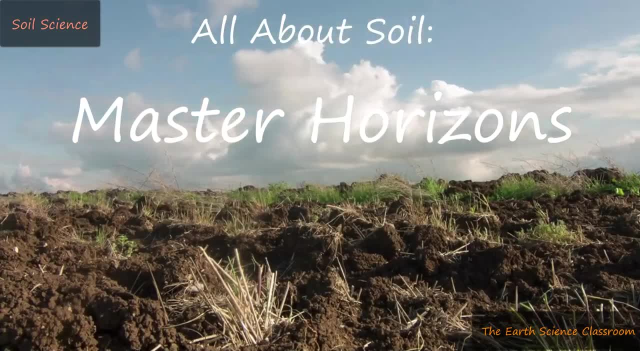 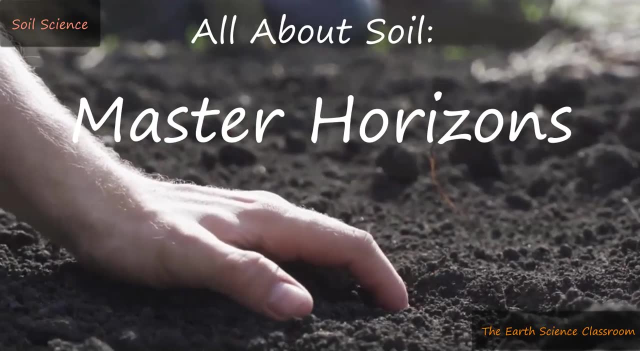 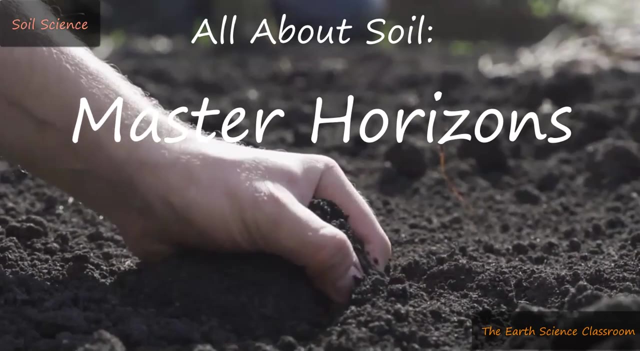 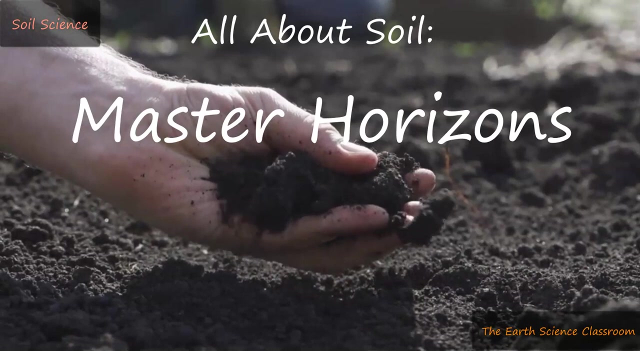 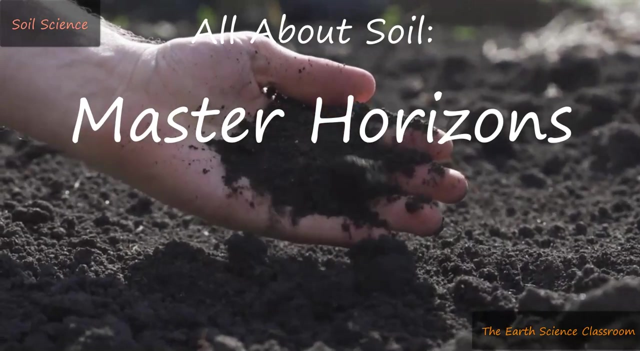 And how soil has played a huge role in making this planet livable, in addition to the other components like the atmosphere and water and the right chemical balances, Right Temperature and the seasons and the tilt and the distance from the sun. But you have this amazing, extremely thin interface which is soil between the rock layers and the surface environment, the conditions on the surface created by climate and location and latitude and elevation. all that good stuff, and how close you are to an ocean. 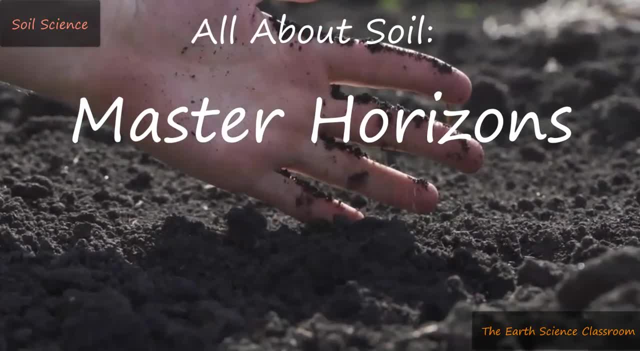 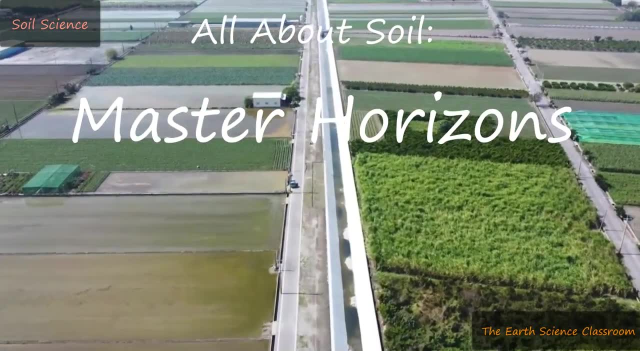 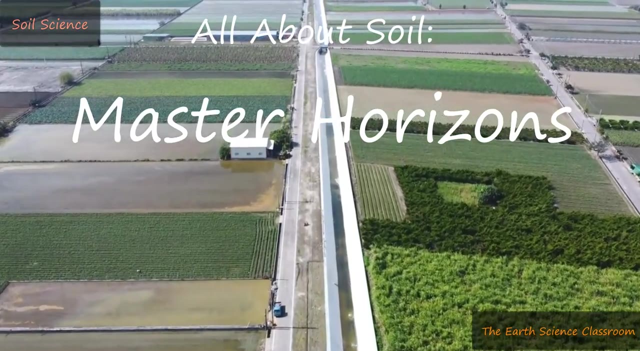 And this thin layer of soil, this top layer of regolith, is single handedly responsible for everything We know of how to feed ourselves and how we get water from the ground, or how we find and cultivate crops and plant life to grow our species into these large societies that we have today. 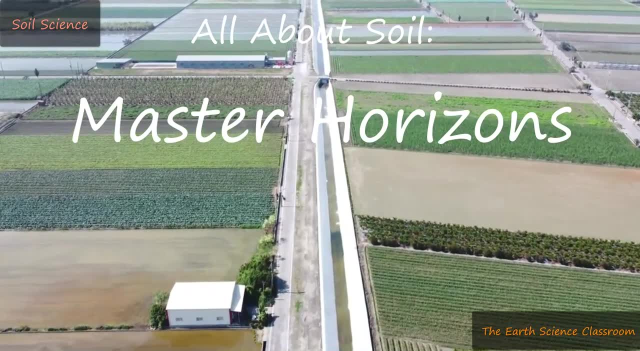 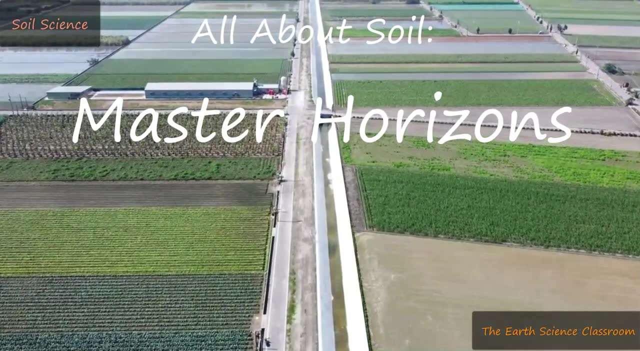 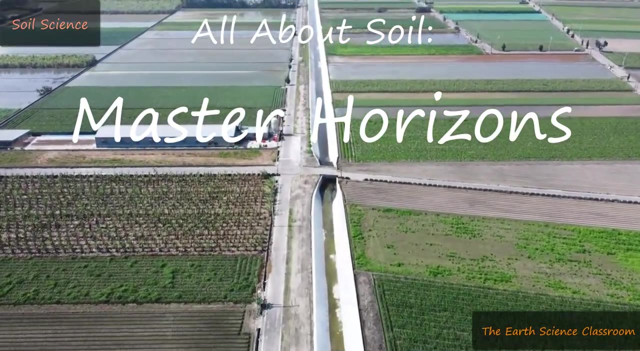 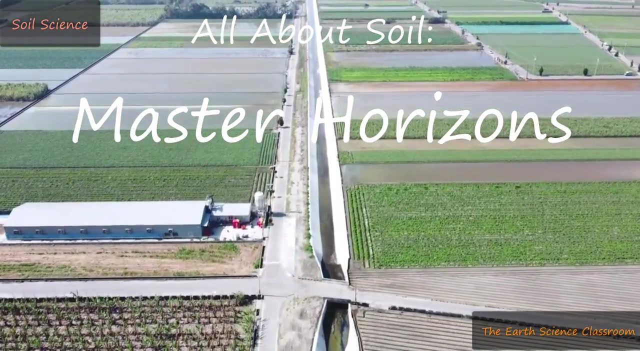 And we built our world around fertile soil, around rivers and flat areas with fertile soil, even around volcanoes. in ancient Italy, around Vesuvius. They knew it was a volcano and had A dangerous component to it, a dangerous aspect, but the soil around Vesuvius was so fertile that they grew all of their crops and their wines and they lived around this, this dangerous natural disaster waiting to happen. 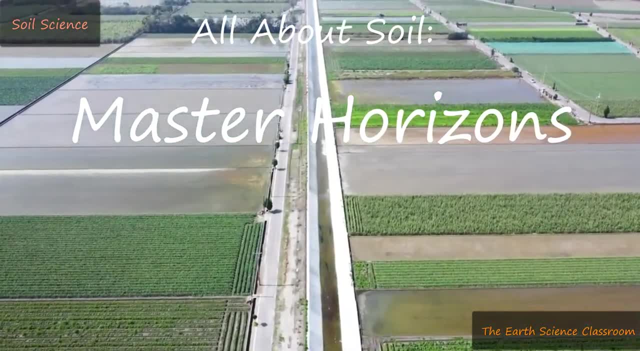 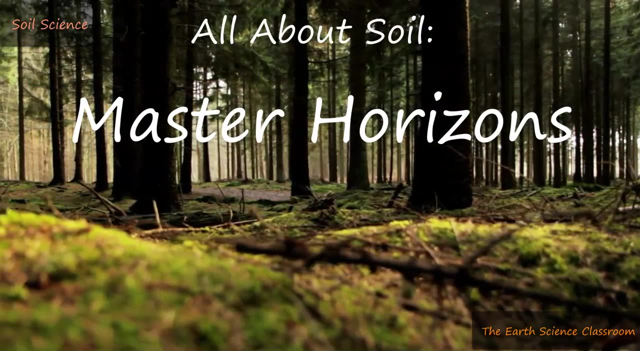 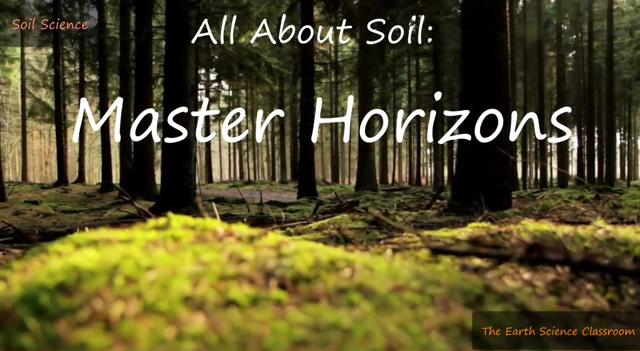 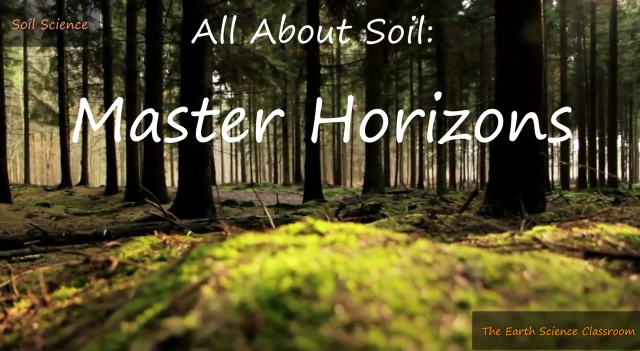 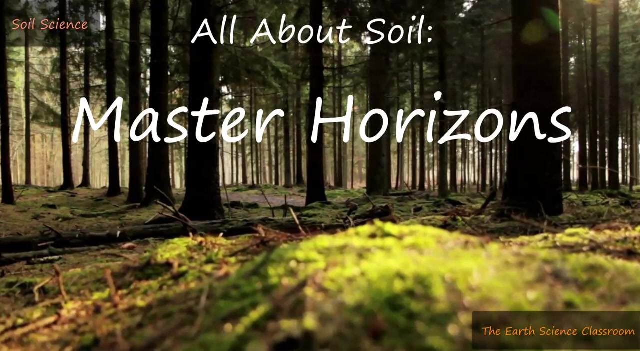 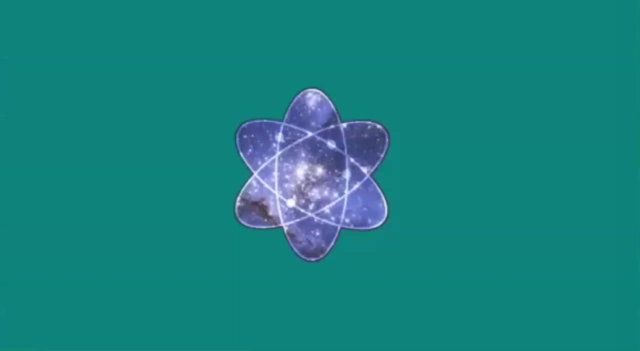 So soil is always a topic that I want to give excitement to, some energy to, because it's so important and so diverse and such a beautiful mixture of all different areas of our planet, both the biological, with the Organisms, both alive and dead. looking at the mixture of the rock and the minerals, then the additional water and roots, and how we use that to cultivate crops and different types of soil, different depths of soil, and to introduce soils as a, as a, as a general term, we're gonna look at what's called the master horizons in this video. 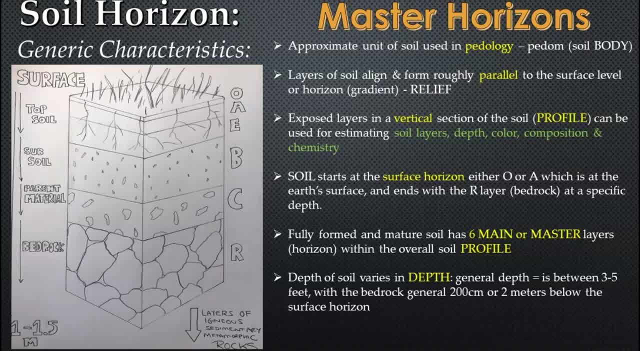 So a master horizon refers to. horizon is a layer, exposed layer of soil underground. so you have your surface, where that may be and whatever landscape and be, and beneath the surface you have these layers of soil and then you go down to a certain depth, usually between three to five feet. one and a half meters down you generally reach solid rock, which is called the bedrock or the R horizon. 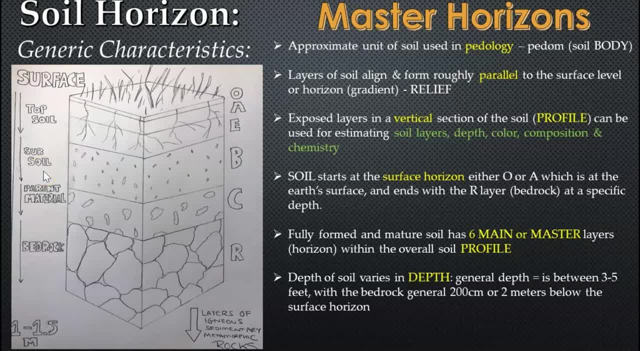 Now the horizon is a layer in the soil. Now each of these layers have Subdivisions and different, different characteristics within them. so the main ones we call master horizons, and there are six in total, and we look at this diagram on the left hand side you'll see up here at the top in this three D very basic drawing is the surface. I personally little grass there or some vegetation or some shrubs, but you have this organic layer up here on the surface called the surface horizon. 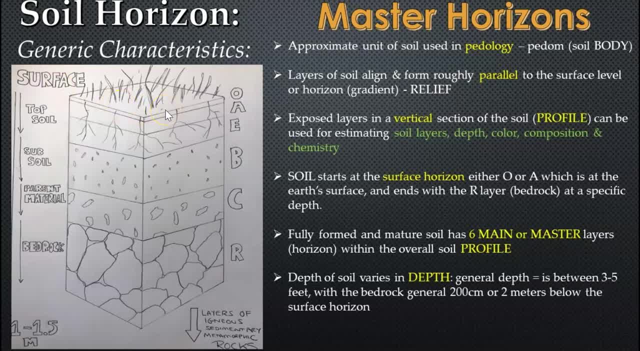 Now, generally, you have some sort of amount of O horizon Which is organic matter, the organic material, and then you have these five or technically four layers or horizons beneath the surface, which is the A, the E, the B and the C. 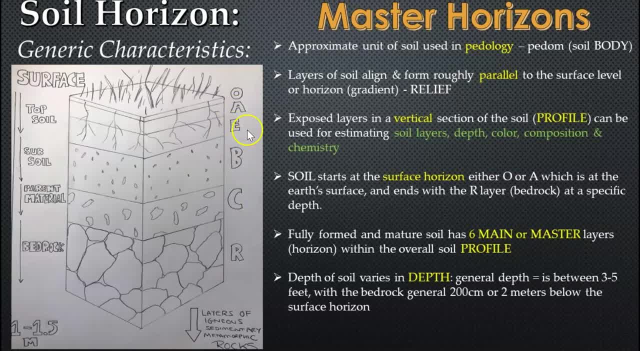 Now it doesn't go in order, though. The E is kind of in between. Now the E comes in a little bit later in the soil formation process or sequential process. You have the A, B and C, A, B and B towards the top, the topsoil, and then you have B, which is a subsoil. 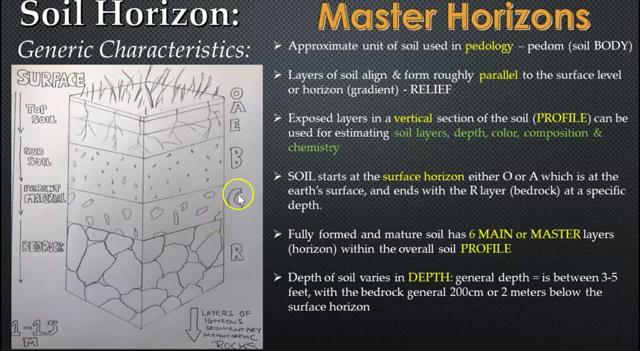 And C, which is down here. it's called a substratum, and that is down towards the bedrock and that contains a lot of the broken bits of material that come from the R horizon. And then beneath this- this is the top of the regolith- beneath the R horizon comes the layers of sedimentary rock, igneous rock and then morphic rock down through the depth of the crust, which could be anything between 10 to 25 kilometers thick, or even thicker on the continental crust versus the oceanic crust. 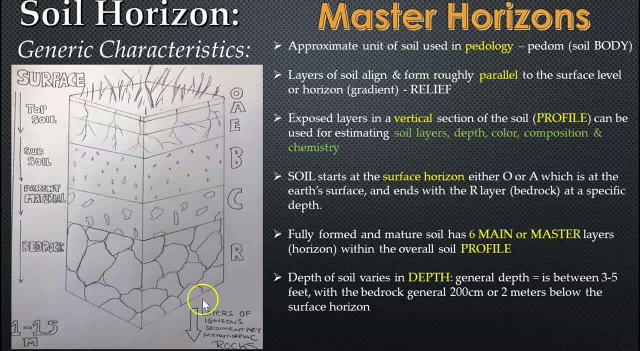 So you have this: You have a vertical profile, a vertical exposed unit of soil starting at the surface where we walk on, and you have these five distinct layers which go down underneath the ground to a certain depth and you'll have water and nutrients and organisms and bacteria and decomposing matter called humus. 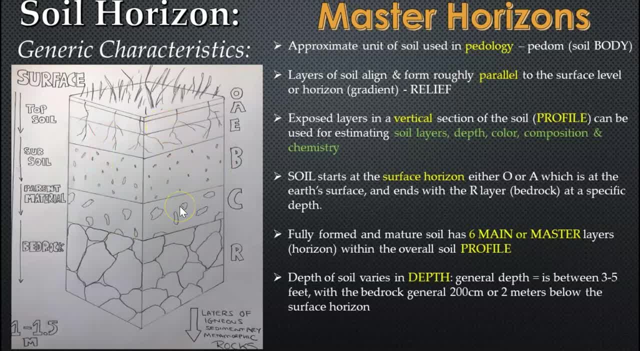 And each layer would have different characteristics and different physical and chemical characteristics which define how we separate These layers into the A, E, B and C. The O one's pretty obvious because that's just organic matter And we can use this profile to establish how fertile or how healthy the soil is, how old the soil is.